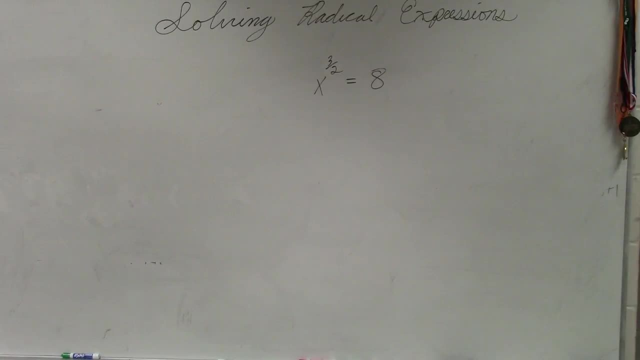 On the next example. ladies and gentlemen, in this case, what we simply have is x to the three halves raised x to the three halves equals eight. Now, ladies and gentlemen, in this example- please take a look here- In this example, when we're looking at this, this is just like last. 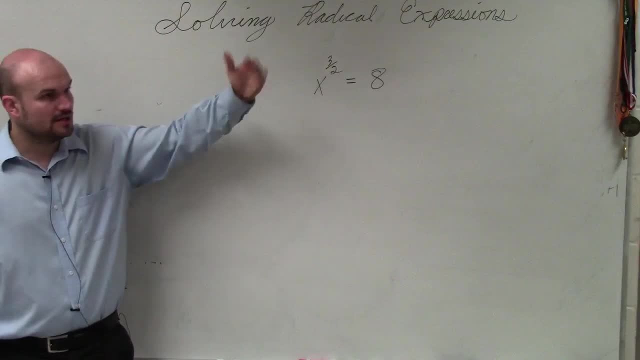 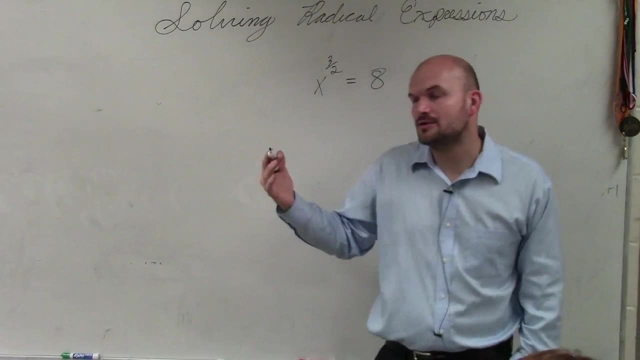 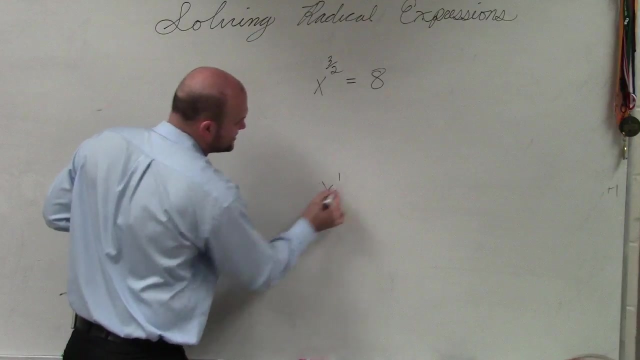 time we used a radical, a radical right, We had the square root. Well, if you guys remember, we can rewrite radicals as our rational root, all right. However, what I'd like you guys to think about this: basically, if we're solving, what we basically want to do is get x to the 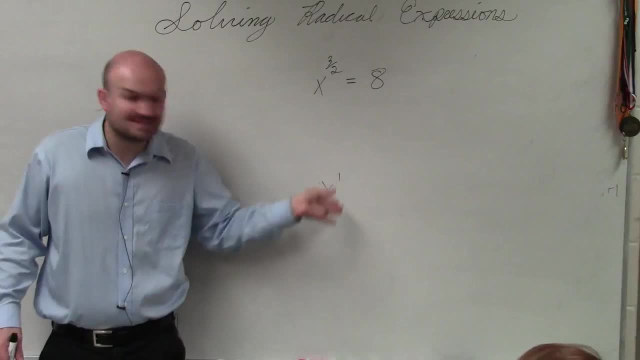 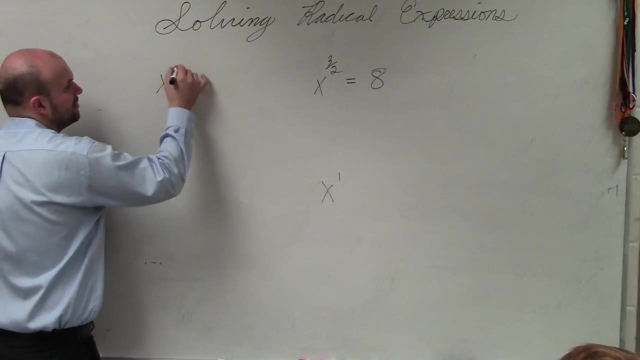 first power. right, We want to solve where x is by itself or when x is to the first power. So, basically, what I want to do is: right now I have x to the three halves And if you guys remember, when we had a variable or a base raised to a power, raised it to another power. 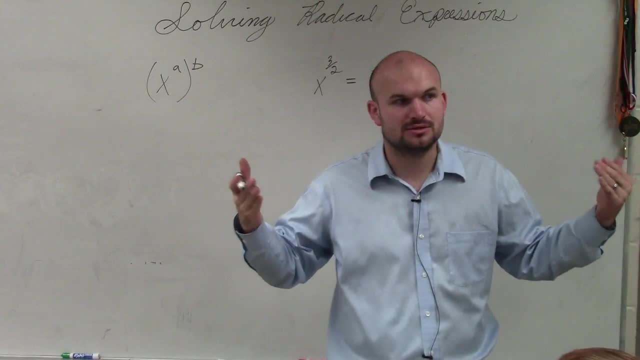 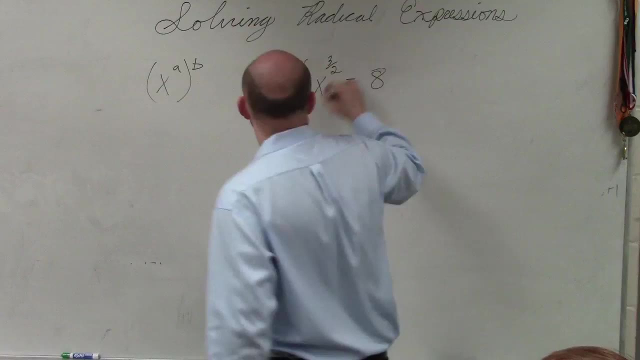 what did we do with a and b? We multiplied them. Whenever you have an exponent raised to a power, you multiply the powers. So what I want to do is I want to raise my x to the three halves to a power that's going to make that one. So what number multiplied by? 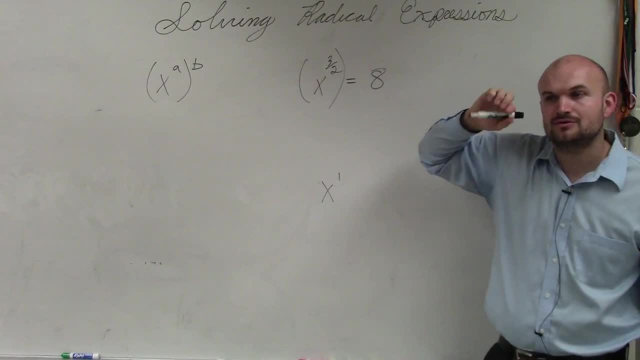 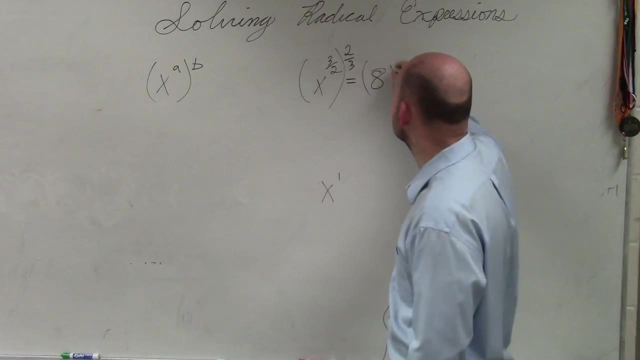 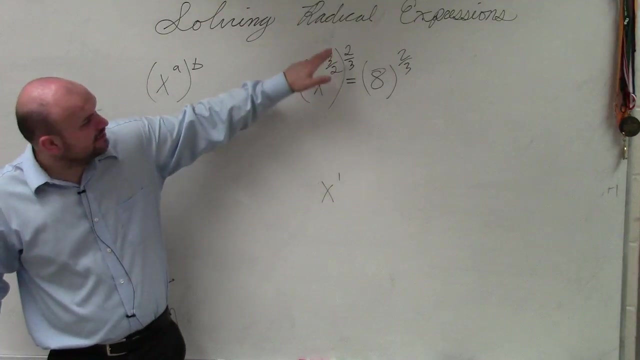 three halves is going to make that one Two over three, which is called the reciprocal. So what we're going to do is we're going to raise both sides to the two-thirds power. okay, See, what happens is you guys can see the three halves, two-thirds, those multiply to give you x to the 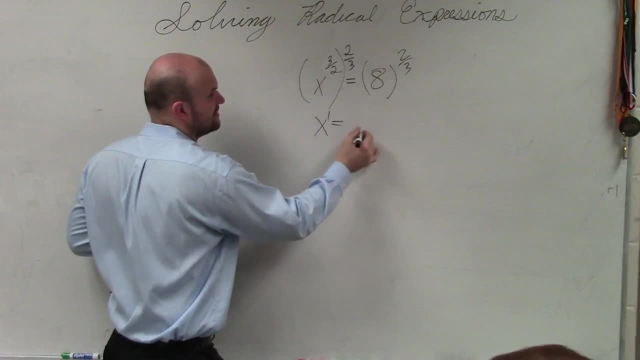 first power. Now I simply just have to do this. I'm going to raise both sides to the two-thirds power. I'm going to raise both sides to the two-thirds power. I'm going to raise both sides to the two-thirds power. 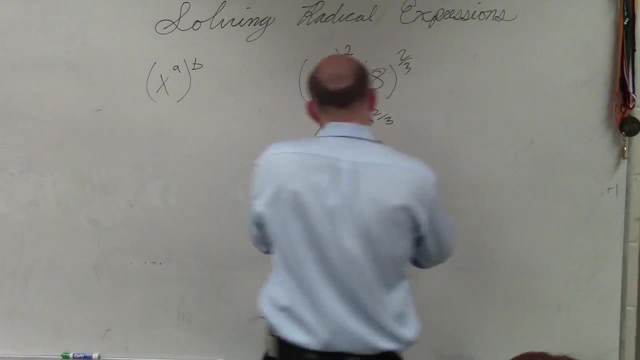 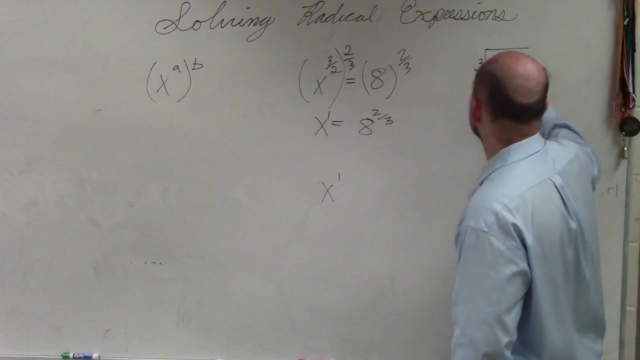 Okay now, there's a couple different ways we can do this. The first way is you guys can rewrite this as a radical expression, which would be the cube root of eight squared. all right, Now, sometimes you guys are going to have some difficult numbers, but if you have a calculator, you can easily go ahead and compute these. 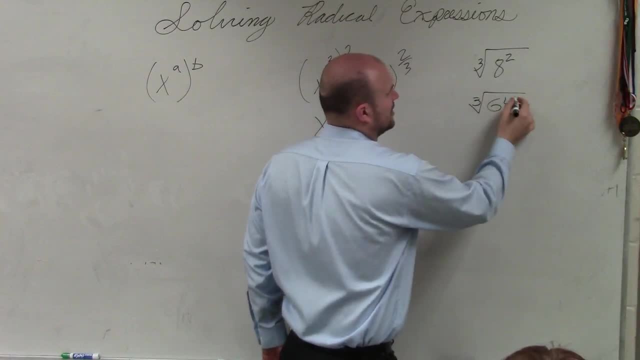 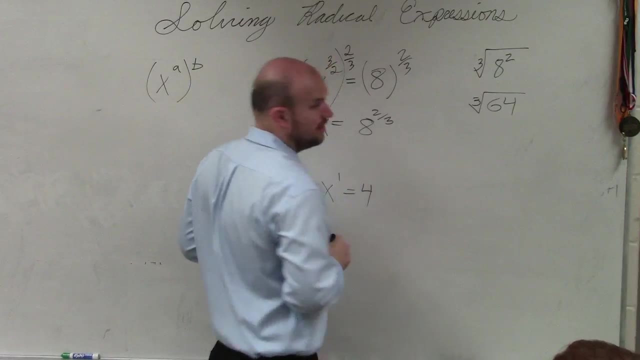 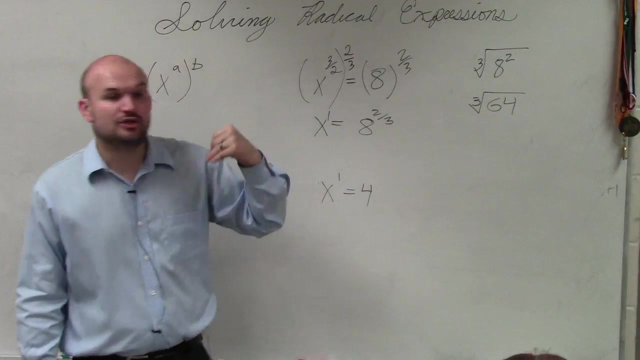 Eight squared is 64.. Cube root of 64, what number, multiplied by itself three times, gives you 64? Anybody know? Eight, Four, Eight times eight is 64.. So square root or square root of 64 is eight, but the cube root is actually four, because four times four times four is 64..